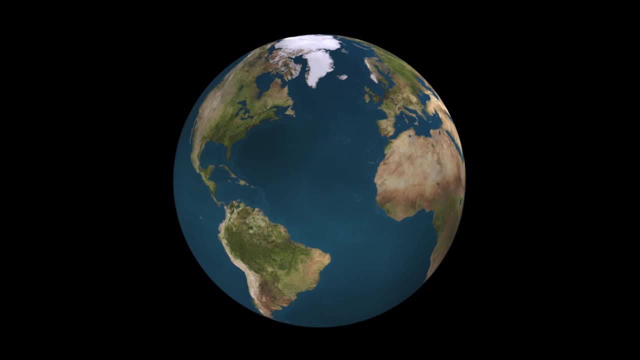 To help us learn about the celestial sphere, let's talk a little bit about how we define locations on Earth, Knowing what we know today: that the Earth is in fact rotating. we can define the rotation axis as piercing through the Earth's north and south poles, and we 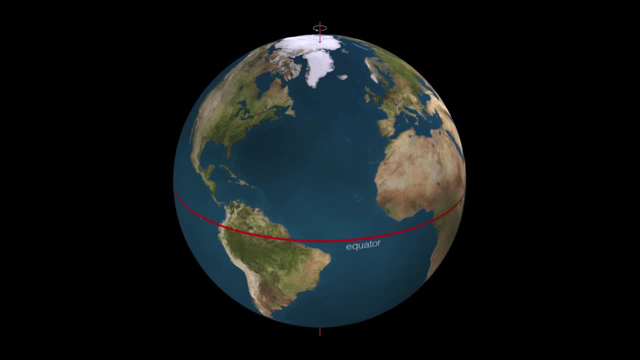 can divide the Earth into northern and southern hemispheres from the equator And we can draw parallels to the equator. So we define the equator as having 0 degrees of latitude, going all the way up to 90 degrees north latitude at the North Pole, And define southern latitudes. 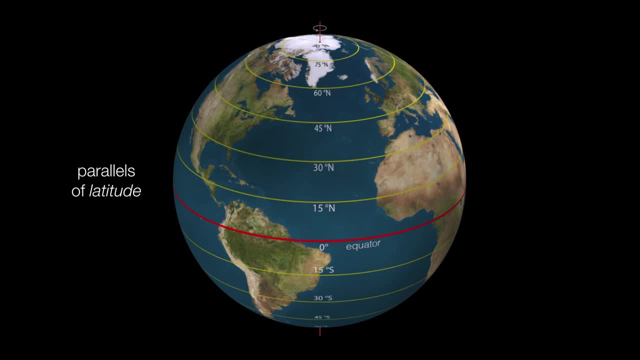 going all the way to 90 degrees south latitude at the South Pole. Most of us live somewhere in between. We can define longitude first by starting off with the prime meridian, which goes from the North Pole through Greenwich, England, to the North Pole through Greenwich. 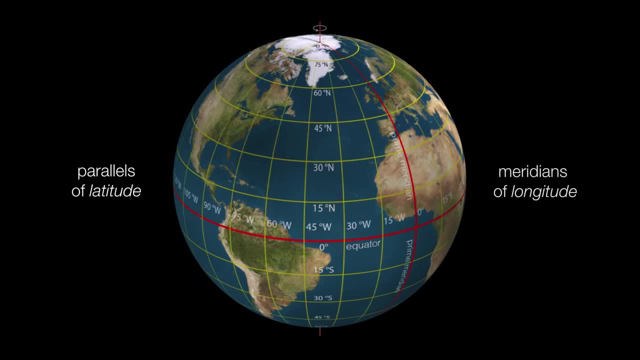 the South Pole and from there we can define what are called meridians of longitude, And this is what divides the Earth into eastern and western hemispheres. So I live near Baltimore. that is somewhere about 39 degrees north latitude and 76 degrees. 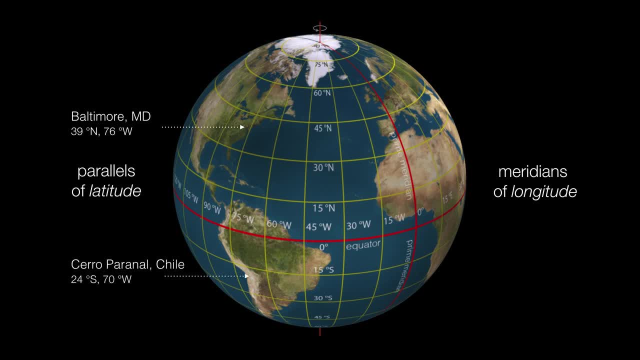 west latitude. The Cerro Paranal, Chile, is home to the European Southern Observatory, and that's at 24 degrees south latitude, 70 degrees west And Rome. Italy, for example, is at 42 degrees north latitude and 12 degrees east. 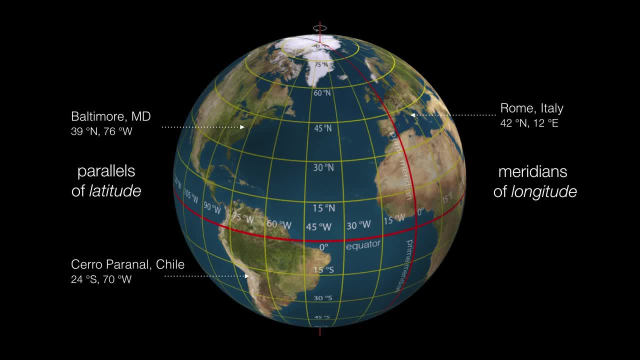 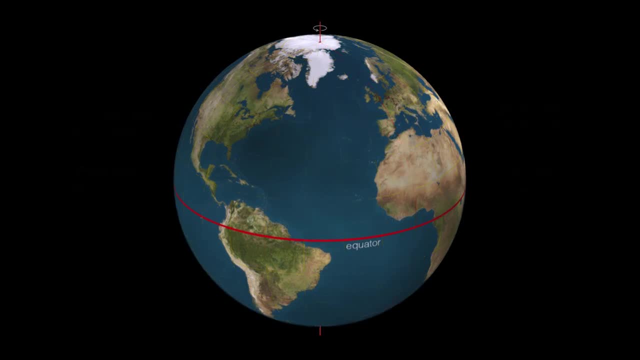 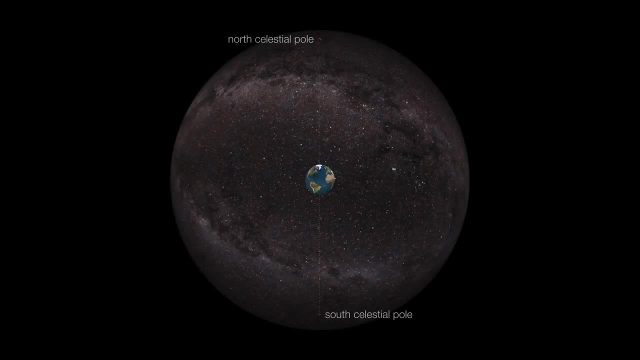 So that puts Rome on the same latitude approximately as Boston Massachusetts in the United States. Okay, well, going back to this idea of the celestial sphere, let's start by taking the Earth's poles and projecting them onto the sky, and that gives us the north and south. 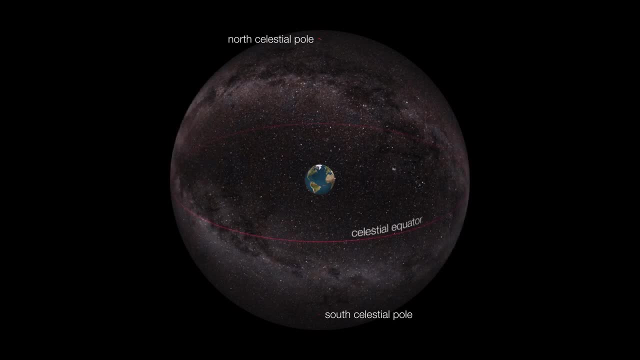 celestial poles And we'll take the Earth's equator And project that onto the sky, giving us the celestial equator. So this in total is the celestial sphere. Now we know today that, no, the stars are not really imprinted on an actual sphere. 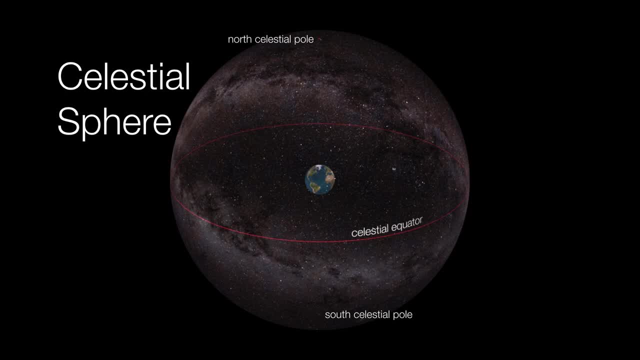 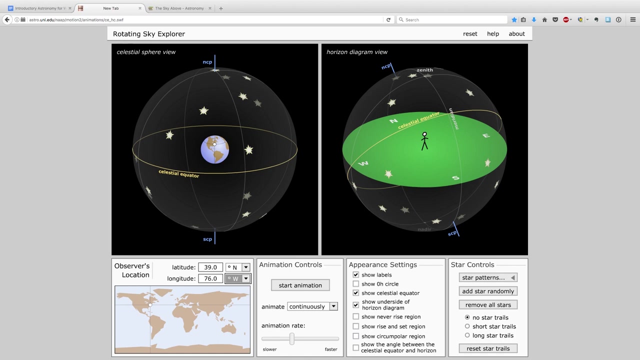 but it's a useful fiction. It allows us to identify not only the positions of stars in the sky, but to help us understand their apparent motion around us. So let's take a look at the sky above us. I've positioned us here in Baltimore, Maryland. 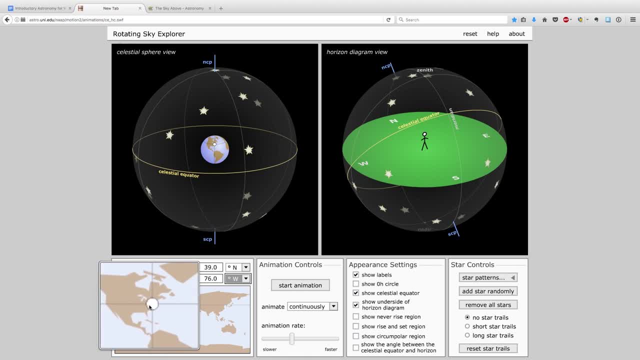 So if you look down here- I've got our location on the map- You'll see that we're at 39 degrees north latitude and about 76 degrees west longitude, And here we are on Earth as well. So we have the north celestial pole and the south celestial pole represented. 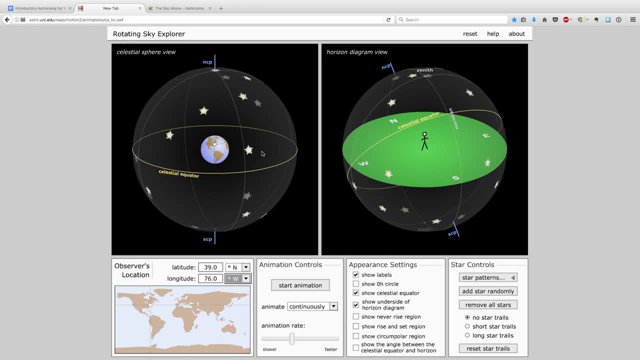 The Earth's equator has been projected onto the sky to give us the celestial equator. So we have the north celestial pole and the south celestial pole represented, And I've gone ahead and just added a few stars at random. On the right side of the diagram is our horizon illustration. 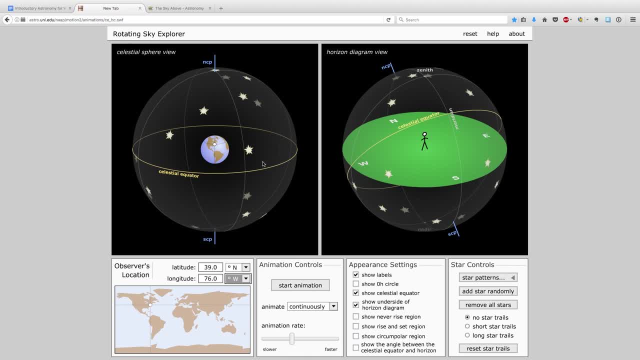 So here we are, standing on our horizon, The celestial equator is projected onto the sky. So the celestial equator is well, I don't want to say visible, because we don't actually see the celestial equator, but it does pass through our sky here in Baltimore. 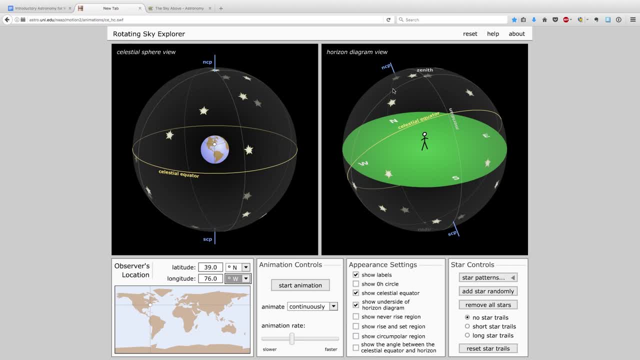 The zenith is directly overhead. The meridian goes from due north through the zenith, So we have the north celestial pole, the south celestial pole, the south celestial pole and the south celestial pole, The zenith, to due south and back around again. 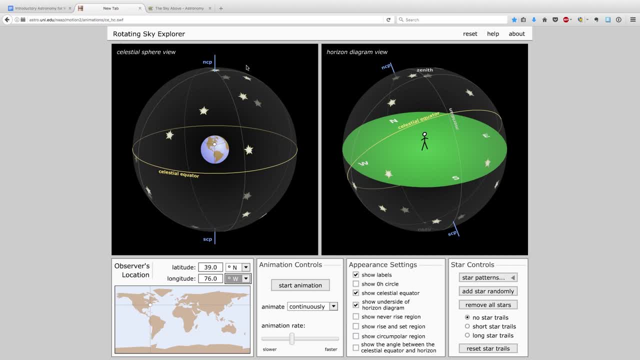 And the nadir is beneath us. So the celestial poles are presented in both diagrams as well, And you notice that the north celestial pole is some altitude above our horizon. Meanwhile the south celestial pole is beneath our horizon, hidden from our view. 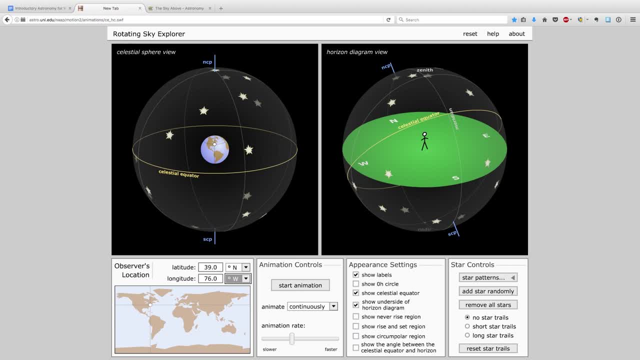 So now let us imagine riding, if you will, along different parts of the Earth, And this is going to help us understand the apparent motion of stars. So let's go ahead and begin our animation, And you'll see that the Earth is rotating. 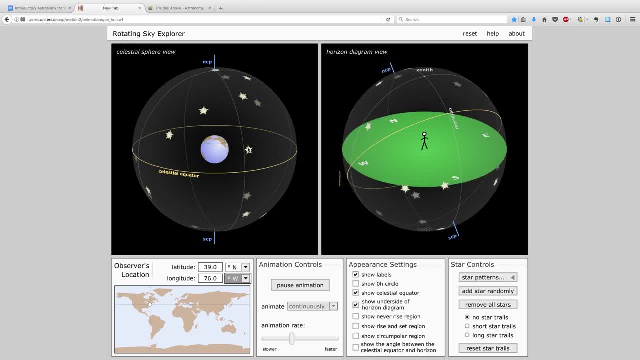 In reality, the stars are fixed, if you will, on the celestial sphere, But from our perspective on the ground, the stars appear to be rising somewhere in the east and, for the most part, setting somewhere in the west. So to help us understand this motion better, 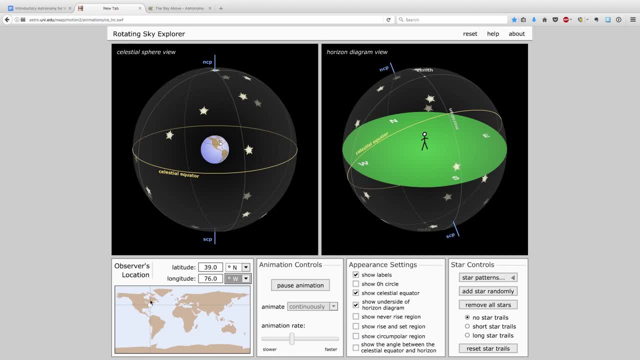 We're going to go ahead and jump from Baltimore all the way to the North Pole. Well, what's going on up here? We're standing at the top of the world, so to speak, and now the North Celestial Pole is directly over our head, at the zenith. 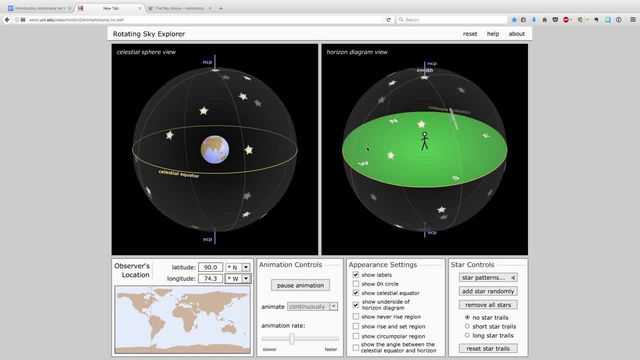 All of the stars in the Northern Celestial Hemisphere are rotating around us. In fact, you notice that none of them are ever setting, None of them are rising. They're just rotating around us carousel style. It's worth noting that only the northern half of the sky is visible. 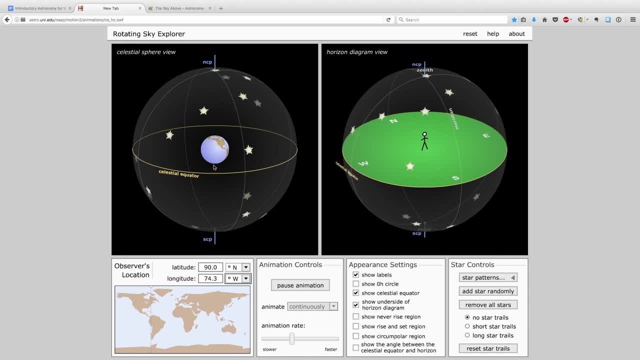 Somebody at the South Pole, by the way, on Earth would likewise see nothing but the southern stars rotating around them. Now let's go ahead and transition from the North Pole down to the equator, So I'm going to set our latitude to zero degrees and notice that once again. 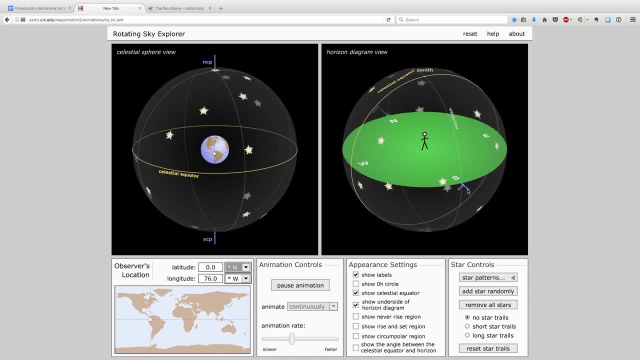 the North Celestial Pole and or the Celestial Poles and the equator. Celestial Equator are still 90 degrees separated from one another as they are seen from this perspective, But because we're at the equator, the Celestial Equator is projected onto the sky directly above. 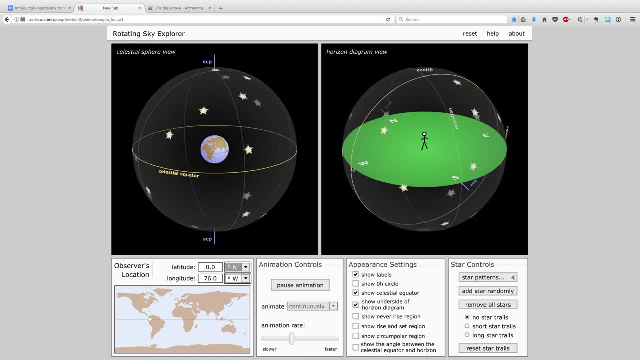 us. In other words, it starts in the east and ends in the west, but unlike what we saw at home, it passes directly through the zenith. Now, what's interesting about this perspective is that, because the North and South Celestial Poles are directly on the horizon, every star in the entire celestial sphere is visible. 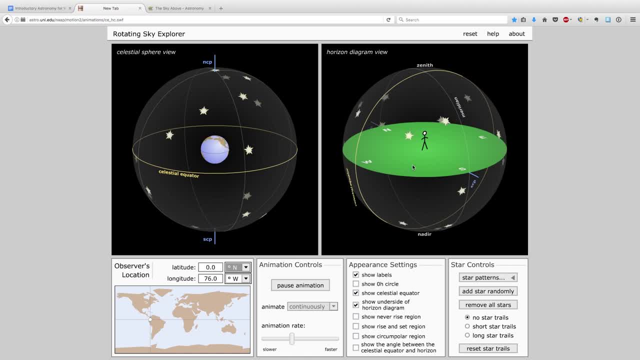 if you are standing at the equator Now, we can't see stars during the daytime. we have the sun out, but different stars become visible at night throughout the year. so that means that throughout the year you will see every star visible from the equator. 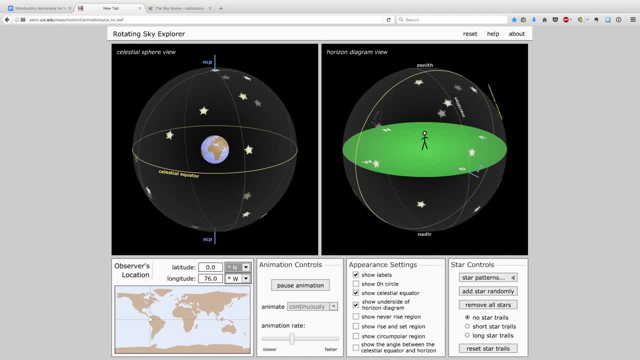 So we can't see stars from anywhere on Earth at the equator. Okay, so what then about those of us who live at mid-latitudes, like most of us do? Let's go ahead and return back home. So go ahead and set us back to approximately our latitude on Earth. and here we are.